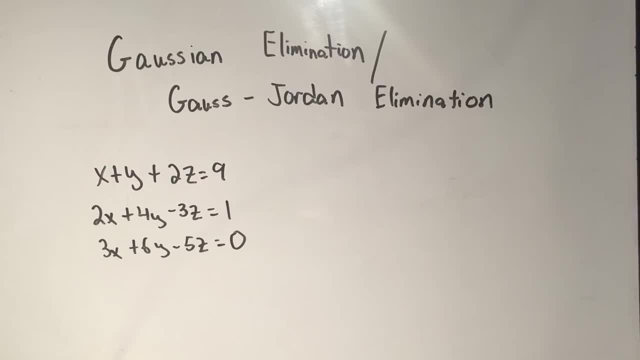 what you learned in say like algebra one or algebra two or something like that. So here I have an example. I've got three equations. I've got x plus y plus 2z equals 9, 2x plus 4y minus. 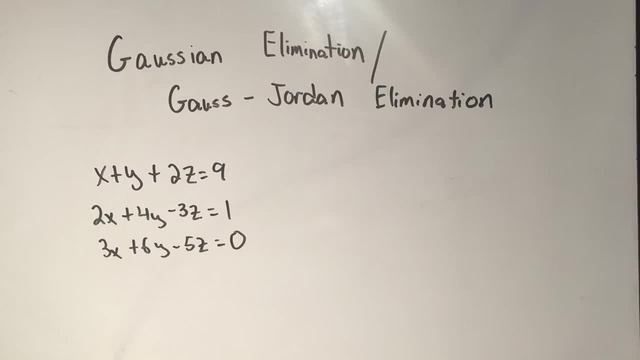 3z equals 1, and 3x plus 6y minus 5z is 0.. And the first thing we're going to do is we're going to put these in a matrix. So I take the coefficients of all these numbers. So the first column is: 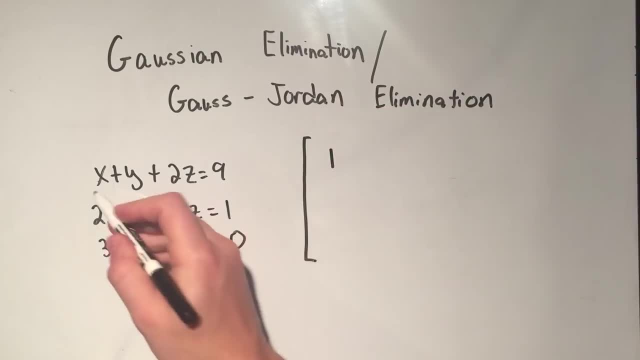 going to be the x column and the coefficients of these are 1,, 2, and 3.. My second column will be the y's, So I take all the coefficients of the y's, that's one, four and six. 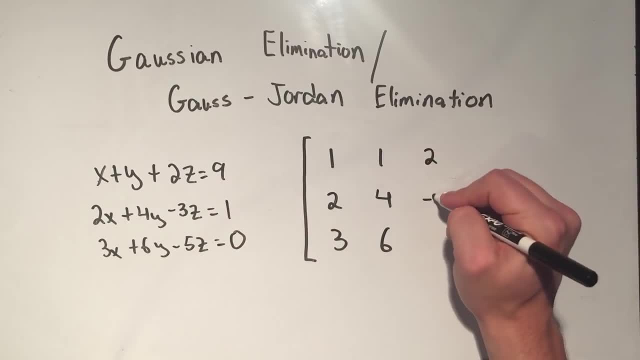 The third column will be the z's, That's two negative three negative five. And then I draw this bar, that's kind of like the equals, and here I put the constants nine, one and zero. So this is called my augmented matrix. 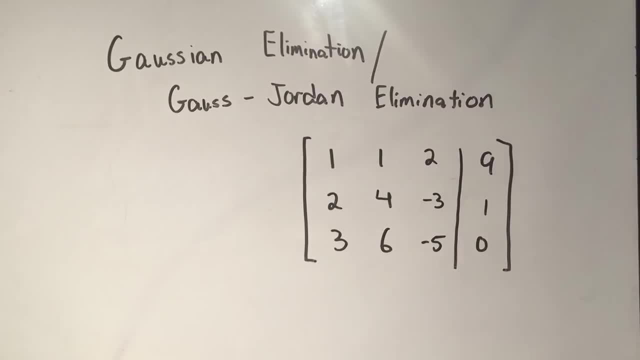 I don't really need this anymore, And now I'm gonna use what are called row operations. So basically, I can add rows to other rows, or I can subtract rows to other rows, or I can multiply rows by a constant or a fraction. 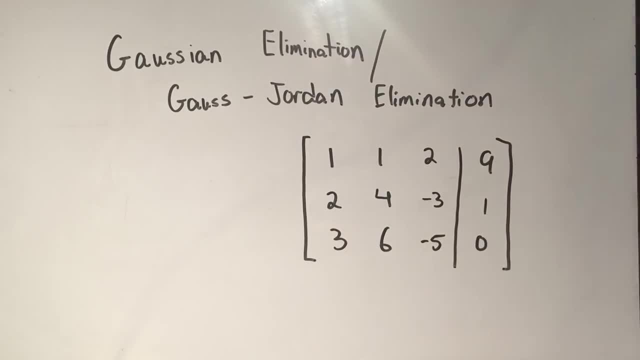 So those are the basic operations I'm going to be using, And my goal for the Gaussian elimination is to get a one and then zeros underneath it. So I'm gonna have a leading one, which is already what I have here, and then zeros underneath. 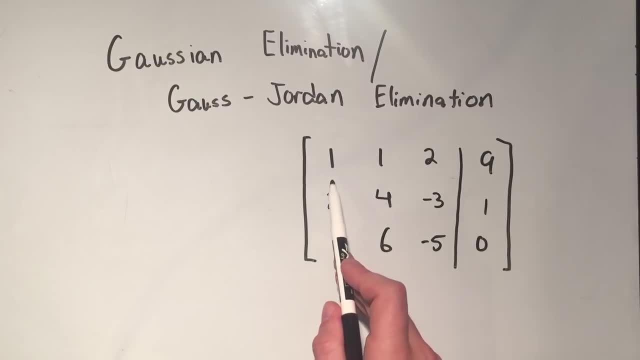 Okay, And then we'll see what happens after that. So right here I already have one, so there's nothing to do, But I want zeros underneath it, So I need to add my first row in some way so that I'll get a zero underneath it. 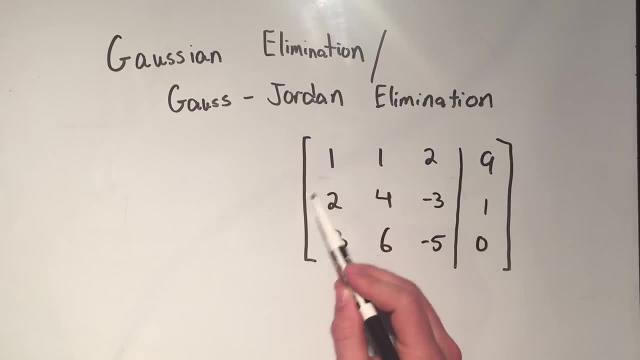 Since this is a one, I need to get it to a two and in fact, I need to get rid of this two. I'm gonna do minus two times row one plus row two becomes my new row two. So this is the notation that you're gonna use. 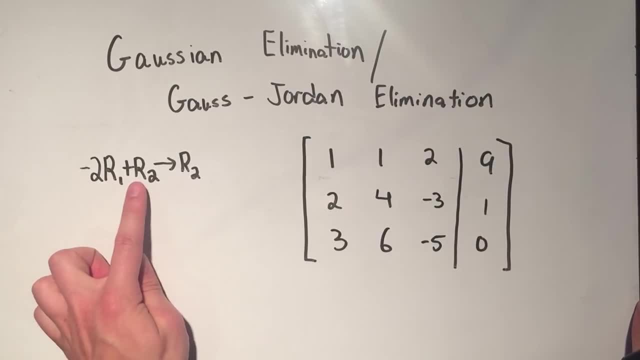 So this says: I have minus twice row one and I'm adding that to row two and that becomes my new row two. All right, So minus two times row two, that would be minus two minus two, minus four minus 18.. So I'm just taking minus two times each of these numbers. 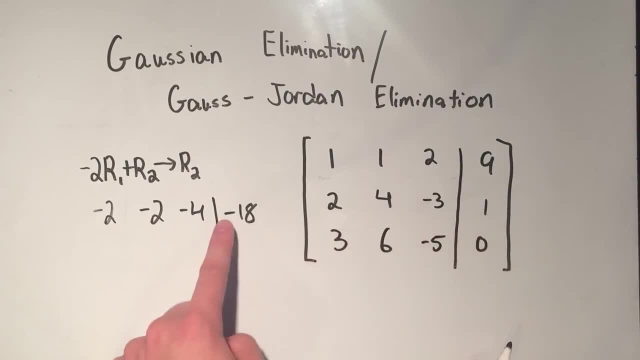 And then if I add these correspondingly, we'll see what happens. So I've got minus two plus two is zero, I've got minus two plus four is two, I've got minus four minus three is minus seven, And I've got minus 18 plus one is minus 17.. 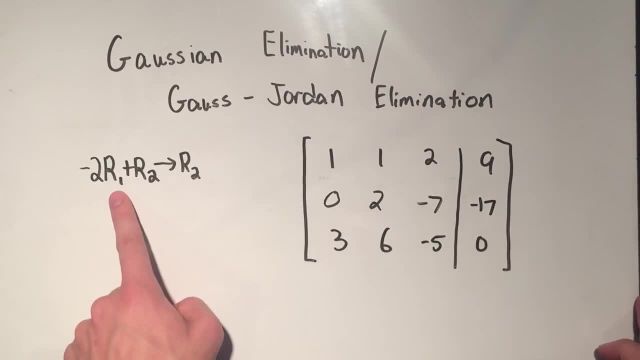 So that was my first operation. So I did minus two times the first row. I added it to the second row, So I've accomplished part of my goal in getting zeros underneath this one. but I want zeros all the way down. So basically I want this three to turn into a zero. 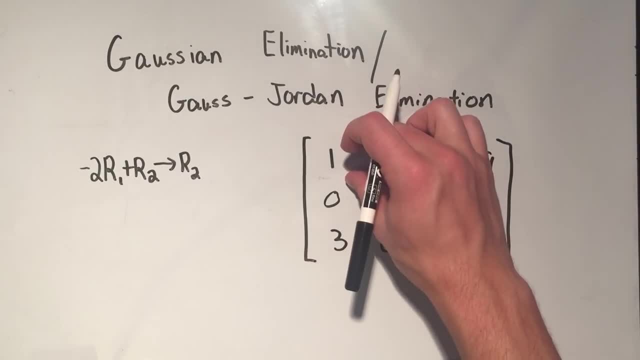 Can you guess how I might do that? Well, I want to take my first row, and this time I'll multiply it by a minus three, so I can add it to my third row, and that will cancel out this three. So that's how I'm picking these numbers. 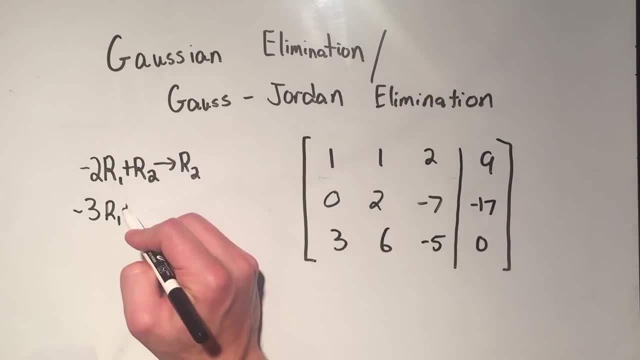 so I can get rid of the numbers right underneath. So if I take minus the first row times three, plus the third row becomes my new third row. So what's minus three, row one? Well, that'll be minus three, minus three. Two times minus three is minus six. 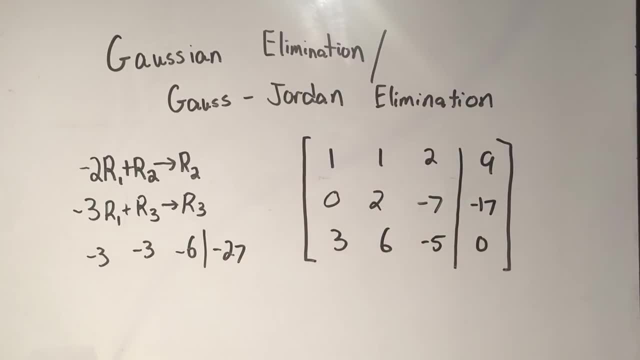 Minus three times nine is minus 27.. And now I'm gonna add this to the third row. I'm gonna add the components together. So I have minus three plus three. that's zero. I have minus six plus or, I'm sorry- minus three plus six is positive three. 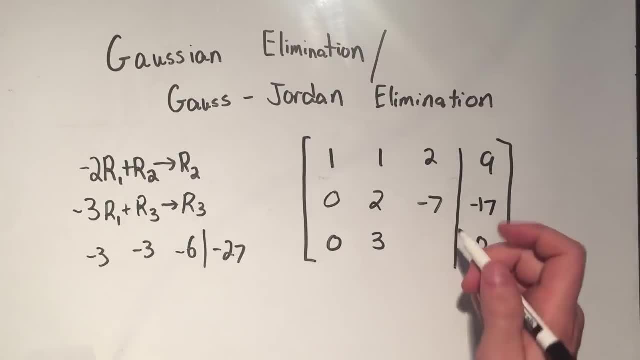 Then I've got minus six minus five, that's minus one Minus 11. And I have minus 27 plus zero is minus 27.. So that's my first step, And now I've accomplished my goal of having zeros below this leading one. 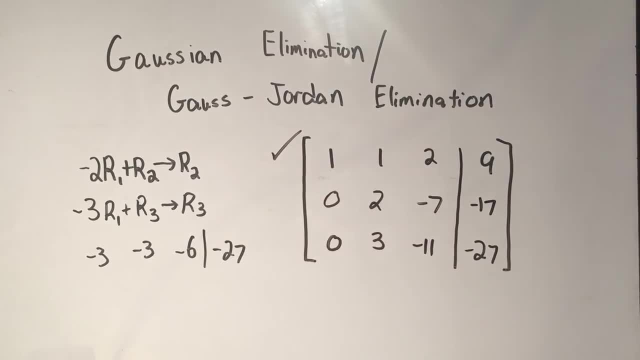 So now what I do? now that this row is done, I move to the second row, And now I want my leading one again. Well, I've got a zero, so that's fine where it is. We already said that was fine. 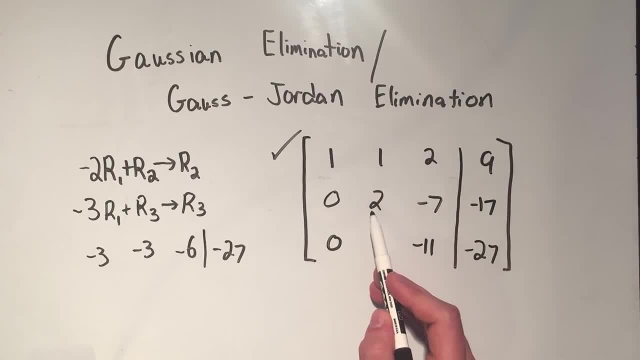 So here's a two. I want this to be a one. I want this two to not be there. I want a one, and then zero is underneath. So I'm gonna take this row and I'm gonna multiply it by a half to get rid of that two. 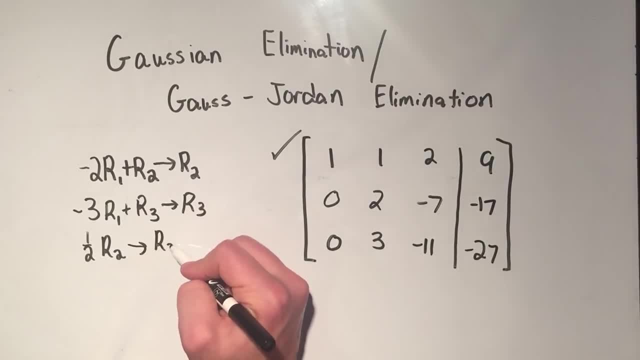 So I take one half of row two and that becomes my new row two. In other words, I'm just dividing each term by two. So that's, two divided by two is one Minus seven. divided by two is minus seven halves Minus 17. divided by two is minus 17 over two. 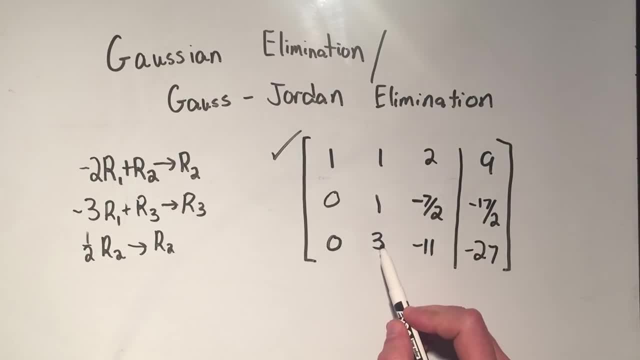 And now what do we do? Well, I want a zero right underneath this, So I need to take minus three times row two. Minus three times row two plus row three becomes my new row three. Notice how I'm using the row right above it. 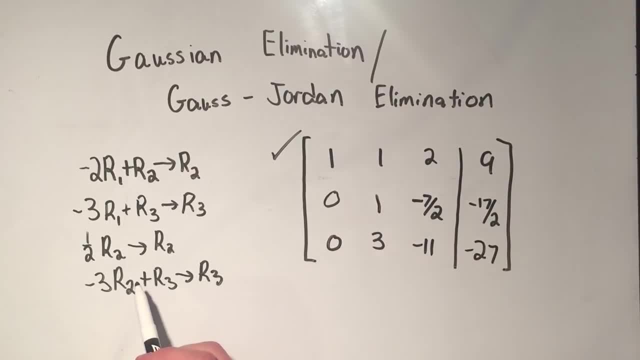 to get rid of the zeros below. So let's look at this. It's gonna get a little involved, but I'm sure you'll be all right. So minus three times zero is zero. I'm not even gonna bother writing it. Minus three times one is minus three. 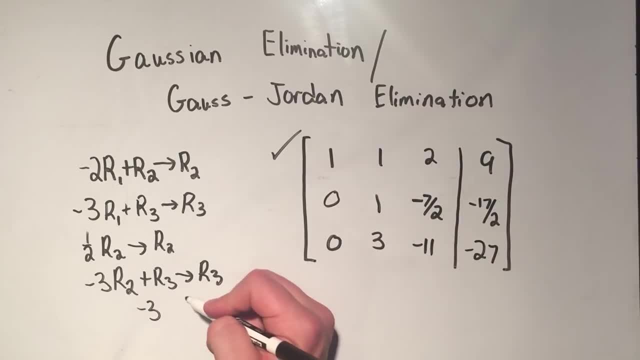 Minus three times minus seven halves. Well, minus and minus is a plus Three times seven is 21 halves Plus five out of seven over here. minus a minus is a plus 3 times 17. let's see: 3 times 10 is 33 times 7 is. 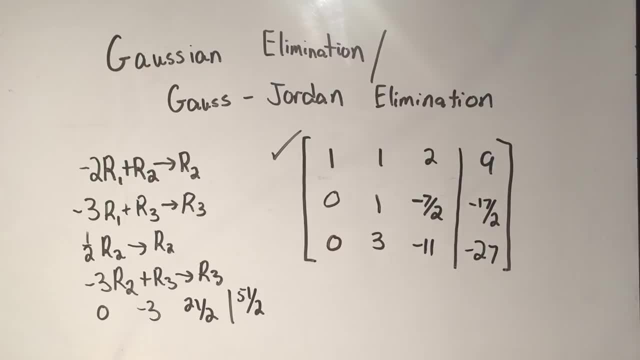 21, I think it's gonna be 51, halves ugly number, sorry. and now it's gonna happen. if I add these component wise, I have: 0 plus 0 is 0, minus 3 plus 3 is 0, and maybe I should change these to over 2 so I can use these fractions. so minus 11 is 22. 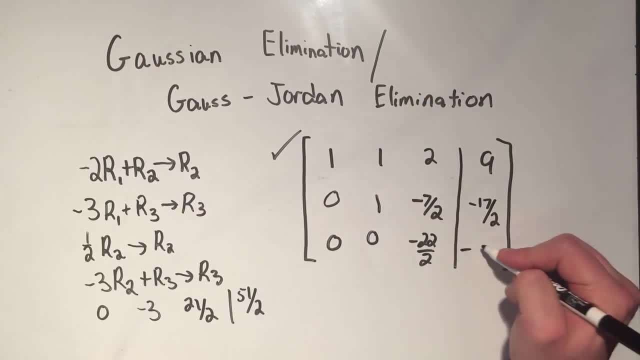 over 2 minus 27 is minus 54 over 2. so I've got 21 over 2 minus 22 over 2, that's minus 1 over 2, and I've got 51 over 2 minus 53. that's minus 72, that's plus 0, that's plus 7xtần, that's minus 33, that's minus. 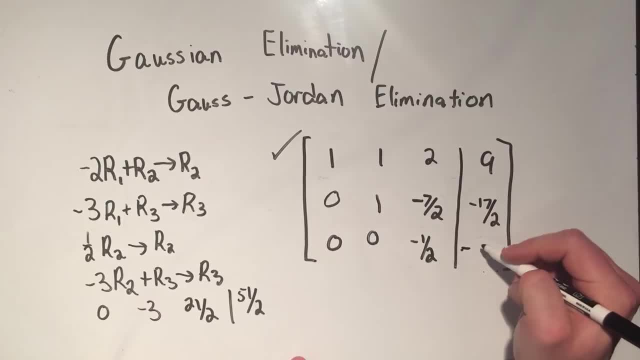 fifty teenagers minus 55- there there are about 3- expands the difference between 54 over 2.. That's minus 3 over 2.. And now I've accomplished my goal of a leading 1 with zeros underneath. Now I go to my very last row. I have 0, 0.. They're good. I want this to. 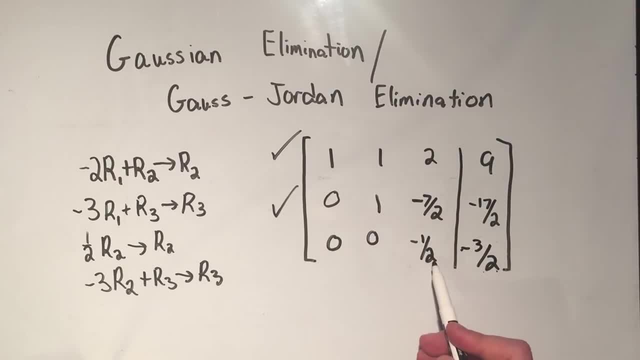 be a 1.. So what do I have to do to get rid of a 1 half? How do I make negative 1 half 1?? Well, if I do minus 2 times row 3, make that my new row 3.. That should do the trick. So if I multiply, 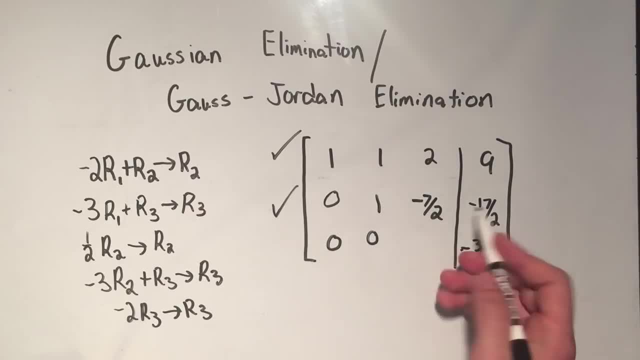 this by minus 2, minus 2 times minus 1 half is 1.. Minus 3 halves times 2 is positive 3.. And now I've got a 1 with zeros underneath. So now this what I've done here: the leading 1s with zeros. 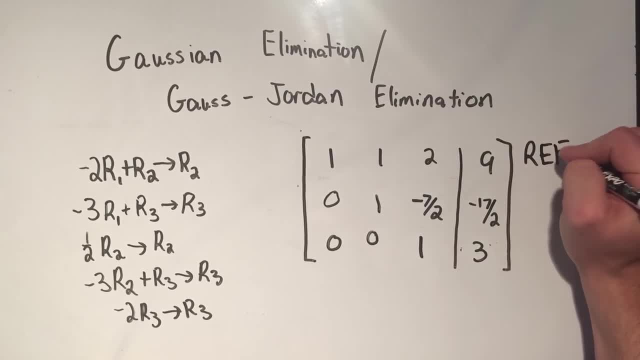 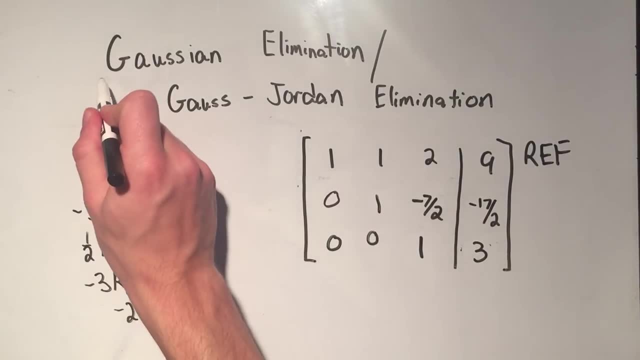 underneath, this is row Echelon form. Okay, I don't know why it's called that, but that's what it's called, And this is as far as you would go with Gaussian elimination. You would put it in row echelon form And you 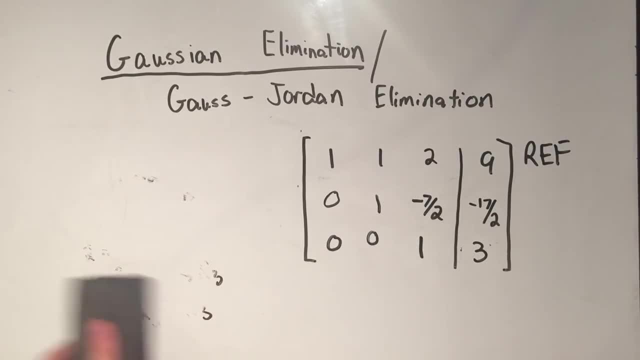 could solve your system like this. So here's how we would solve the system. I look here. I basically have 0x plus 0y plus 1z equals 3.. And this simply means that z equals 3.. I can just read the answer. I've got 1z equals 3.. Let me look at my second equation. I've got 0x. 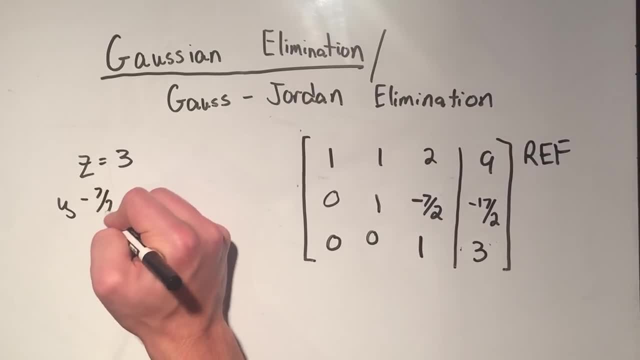 plus 1y minus 7 halves. z equals minus 17 halves, But I just found out that z was 3.. So let me plug 3 in for z. That's y minus 7 halves times 3 equals minus 17 halves. 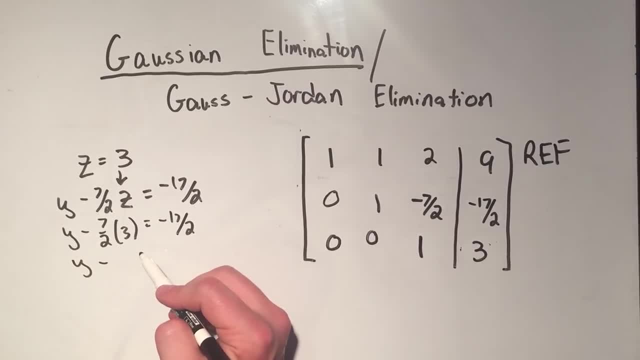 That's y 3 times 7 is 21 halves, equals minus 17 halves. And now if I add 21 halves over minus 17 plus 21 is 4 halves or 2.. So I know that y equals 2.. And then I look at my very first equation. 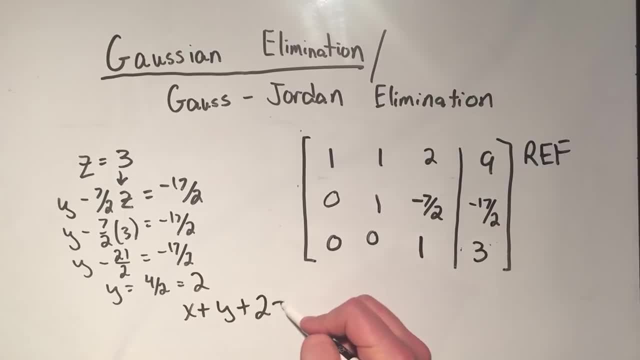 I've got x, 1x plus 1y plus 2z, equals 9.. But I know that z is 0x plus 1y plus 2z, equals 9. And I think I solved this just like I did And I. 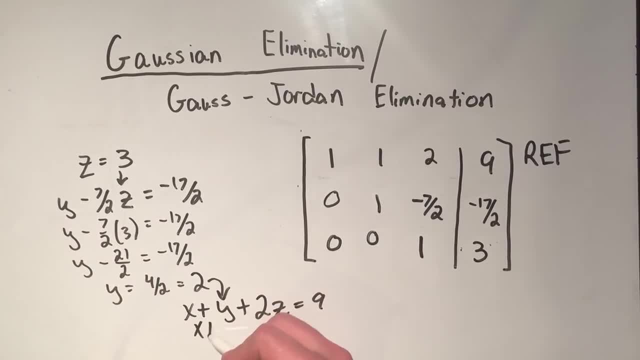 what Y is. Y is 2, 2 Z. I know what Z is. Z is 3, which means that X equals. let's see, I've got 9 minus 2 times 3 is 6 minus 2. it's gonna be 3 minus 2, I think that's. 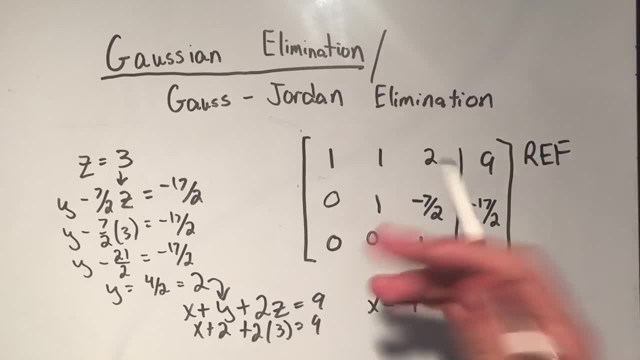 gonna be 1. yes, okay, and there you have it. you've solved the system of equations using Gaussian elimination. so you see how that works. we got these leading ones, we got rid of everything underneath, so there were zeros under the leading ones. and then I did this back substitution thing. I started from the bottom and I 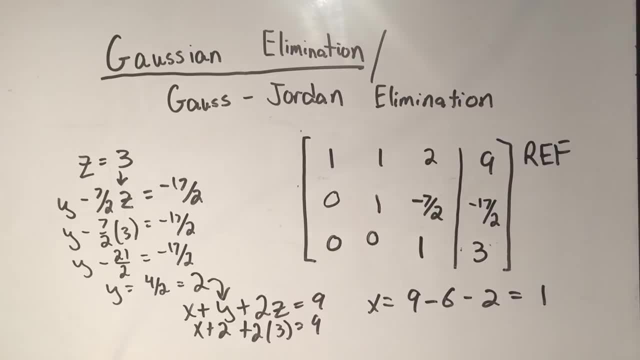 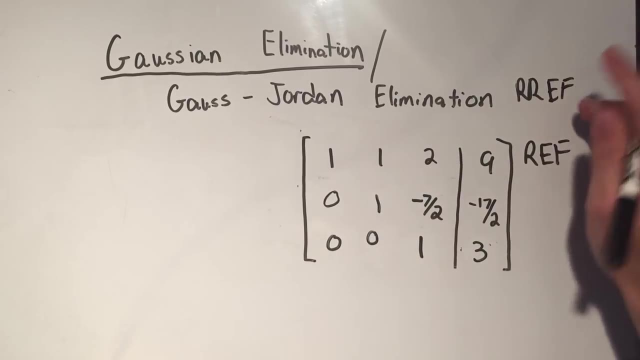 substituted. I solved the second equation and I substituted to get the first equation, that's Gaussian elimination. but if you want to do Gauss Jordan elimination, we want to put it in reduced row echelon form. so this is row echelon form. Gauss Jordan is reduced row echelon. 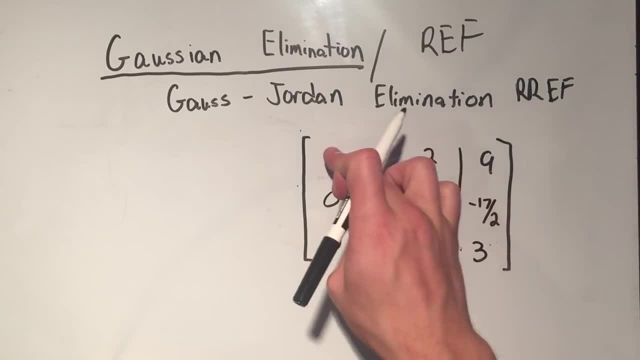 form and what that is is that's just ones along the diagonal and zeros everywhere else. so I'm kind of kind of do the same thing, but I'm just gonna be using the matrix. I'm not gonna be doing using equations and substituting. so, just like I got zeros underneath the ones, now I 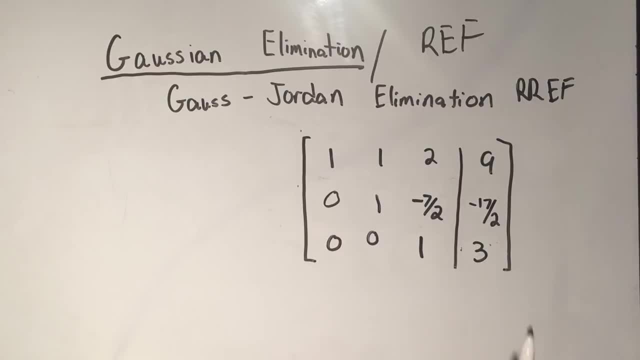 got zeros above the ones as well. so now I start with my third row and I think: what can I? how can I add my third row to my second row so that there's a zero right here? well, since this is already a 1, if I take 7 halves times my row 3 and 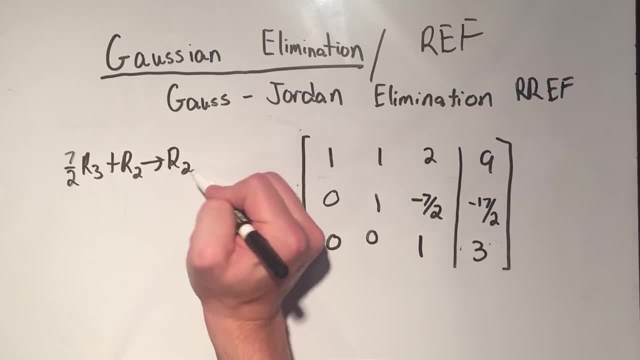 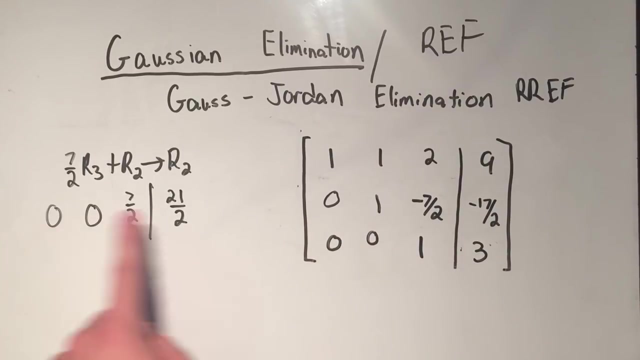 I add it to my row 2 to make that my new row 2. that should cancel the thing out right above, because I've got zero, zero. seven halves times 1 is seven halves, and then seven halves times three is twenty one-half. and now i add this to my second row: 0-plus. 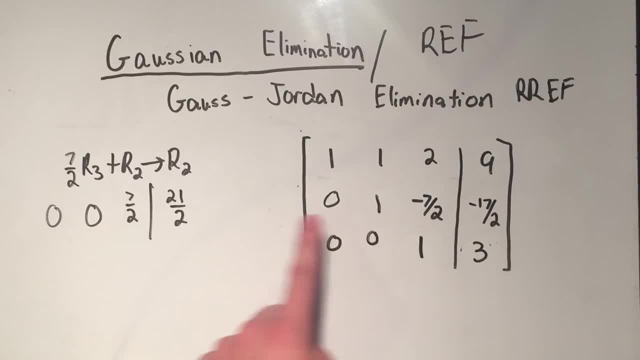 zero is 00 plus one is 1,. 7-halves minus seven-halves is 0, as desired. and then twenty one over two minus 17 over 2.. That's 4 over 2. And we found that to be 2.. And would you look at that? I can already read. 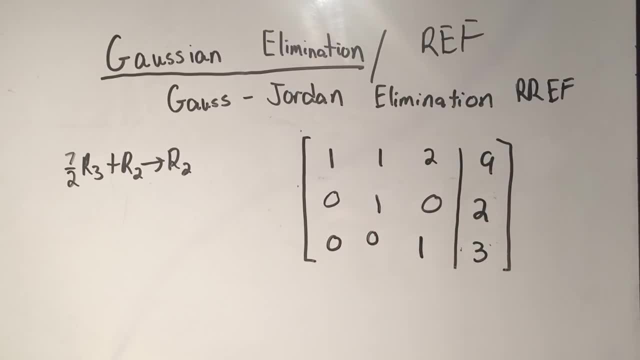 that y equals 2,, just like we found using Gaussian elimination. And now I'm going to do almost the same thing. I'm going to have to use the third row and the second row and add it to the first row to get rid of the 0, or to get rid of this number and this number, So to use the third row to get rid of. 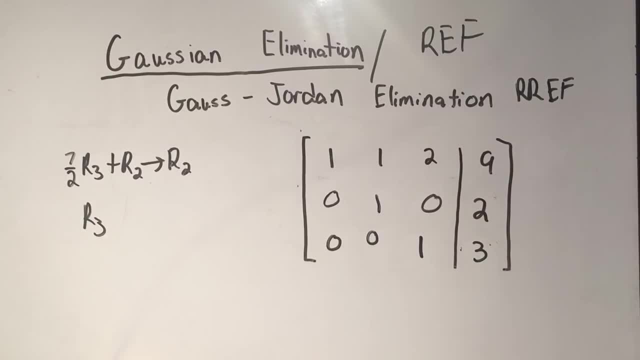 this 2, since I want 0s all the way up, I'm going to have to do 2 times row 3,, in fact, minus 2 times row 3,, add it to row 1, and that'll be my new row 1.. So, minus 2 times my third row, that's 0, 0,. 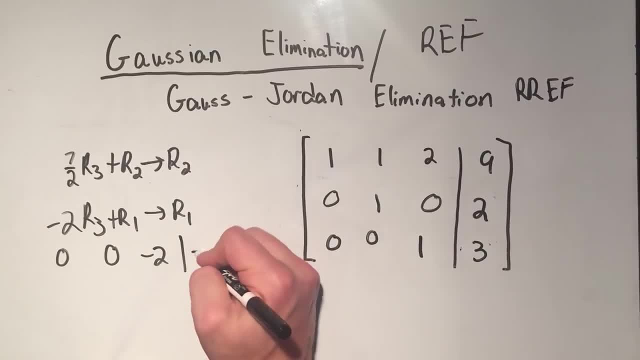 minus 2, minus 2 times 3 is minus 6.. And now, if I add this to my first row, 0 plus 1 is 1, 0 plus 1 is 1, minus 2 plus 2. 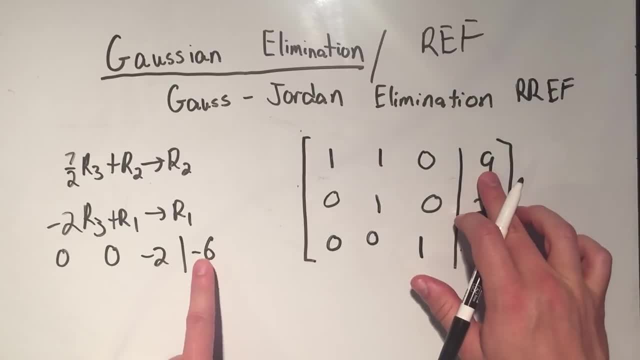 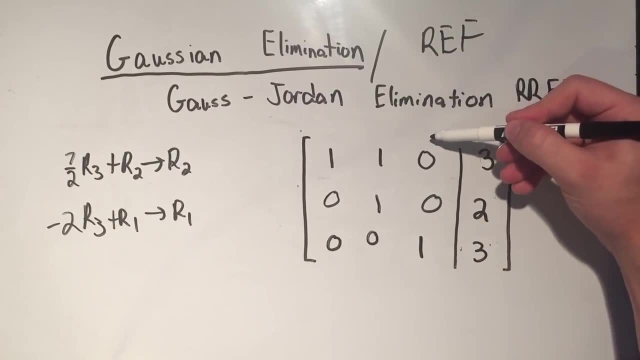 is 0, and then minus 6 plus 9 is 3.. We're almost done Now that I have 0s completely above this one. I just need a 0 above this one right here, So I'm just going to take minus row. 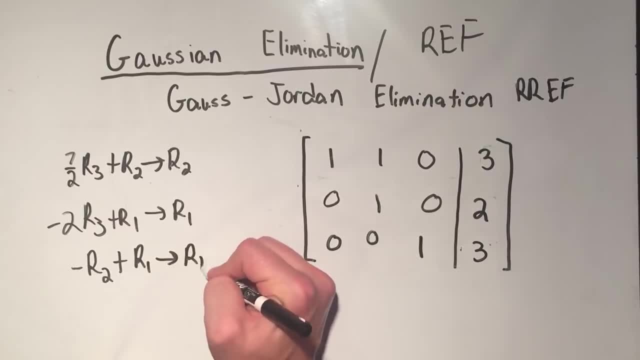 2 plus row 1 to give me my new row 1.. And now I'm just adding the negative this to this, so that's 0, minus 1, 0, minus 2.. If I add this to this, 0 plus 1 is 1, minus 1 plus 1 is 0,. 0 plus 0 is 0,.